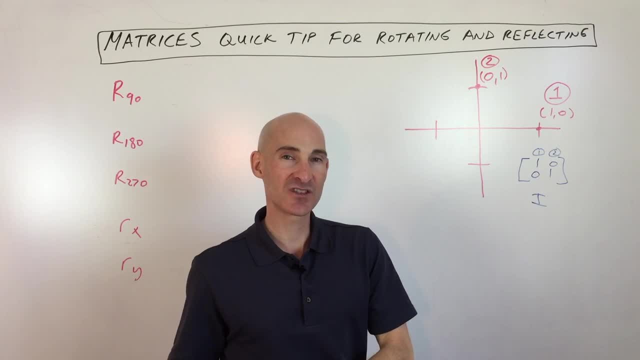 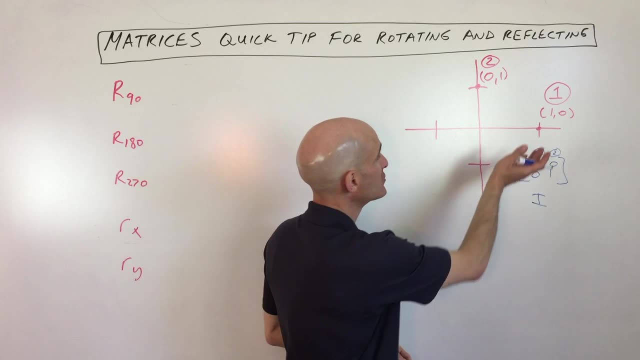 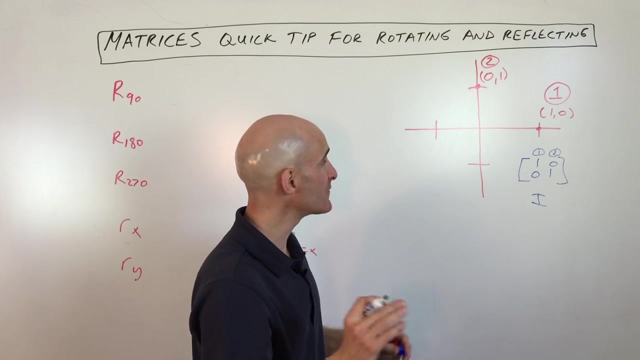 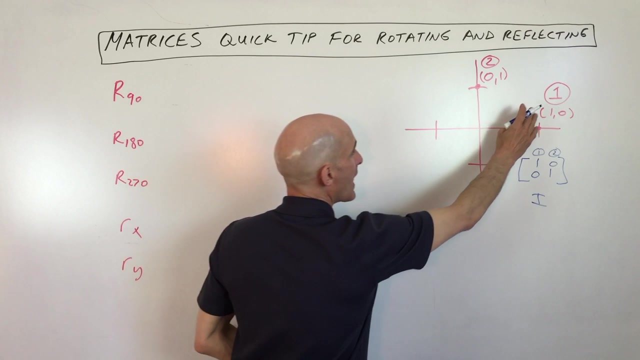 matrix back. So it's just like multiplying by the number one. Anything times one gives you itself back. Same thing with the identity matrix, And what we're going to do now is we're going to look at how does this matrix change as you rotate 90 degrees, 180,, 270, and if you reflect over the x-axis, y-axis, or the line y equals x. It's very easy. All you do is pay attention to these two points. If we want to remember the matrix that rotates 90 degrees, we look at what happens to point one and two when we rotate 90. So if we rotate 90, okay. 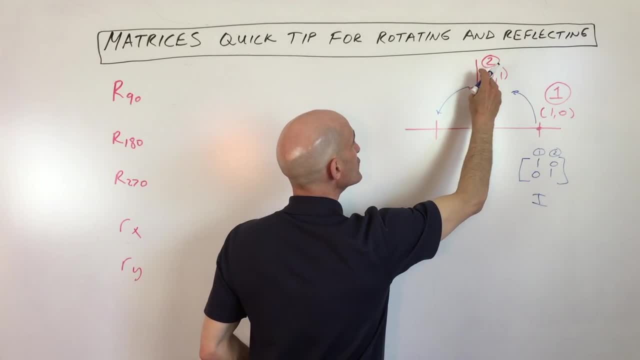 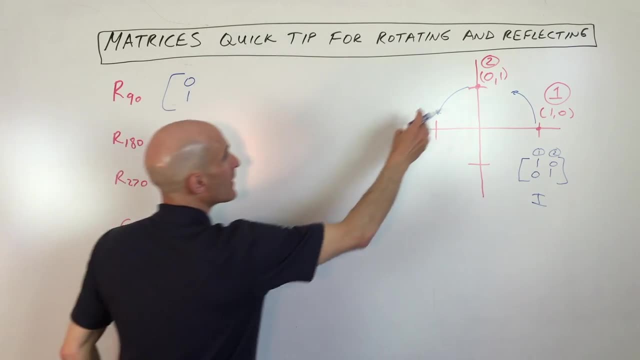 look at what happens. Point 1, 0 moves to 0, 1.. So what I'm going to do is I'm going to replace point one here with its new coordinates 0, 1.. Point number two- 0, 1, is going to move to this. 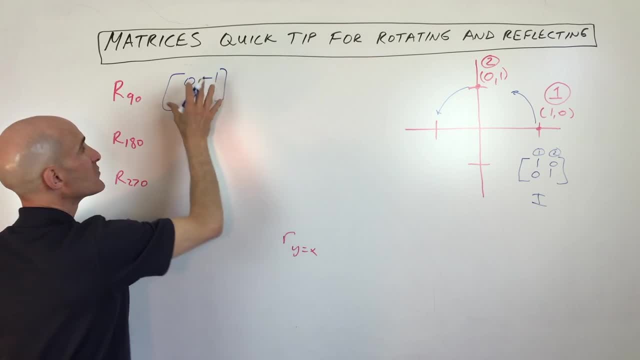 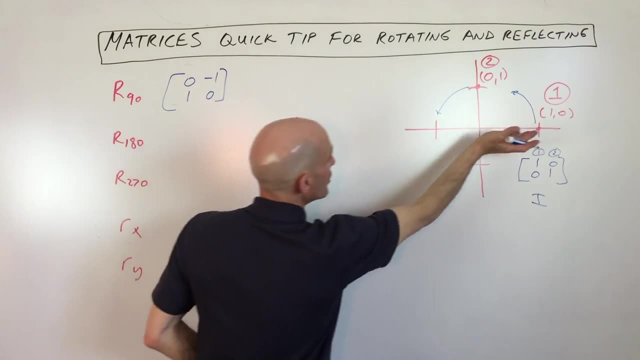 point over here which is negative: 1, 0.. So this matrix is going to be the matrix we want. if we want to rotate 90 degrees, Okay, let's look at 180.. So if we rotate 180, this point is going to. 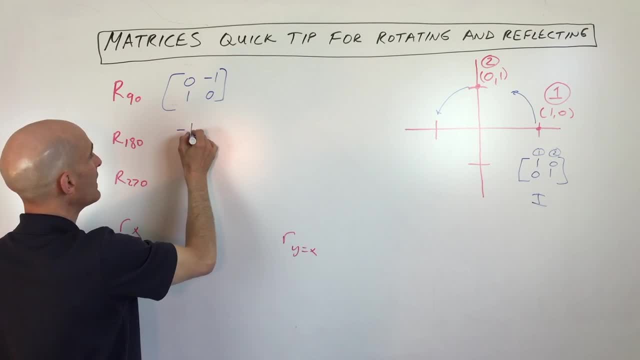 move half a rotation over to here, which is going to put us at negative 1, 0, whereas point number two is going to rotate all the way down to here, and that's a coordinate that's going to be 0, negative 1.. So by multiplying by this matrix, you're going to be able to rotate, you know. 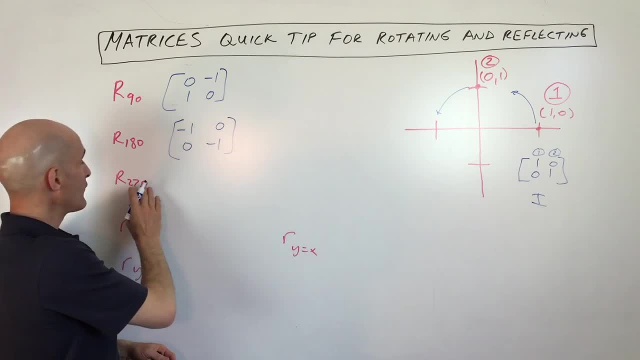 a preimage to its image: 180 degrees. If you rotate 270, this point here is going to rotate three quarters of a turn. It's going to end up at 0, negative 1, and this point- 0, 1, is going. 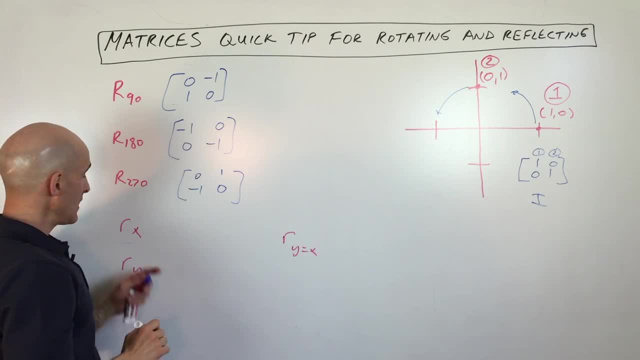 to rotate three quarters of a turn. It'll be at 1, 0.. Now if you reflect over the x-axis, we're folding it over the x-axis, the mirror image. this point is actually on the line of reflection. so 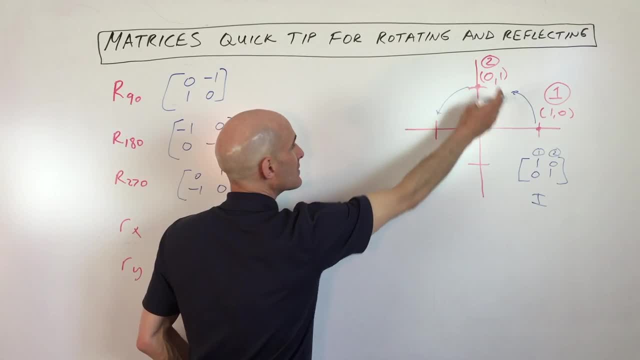 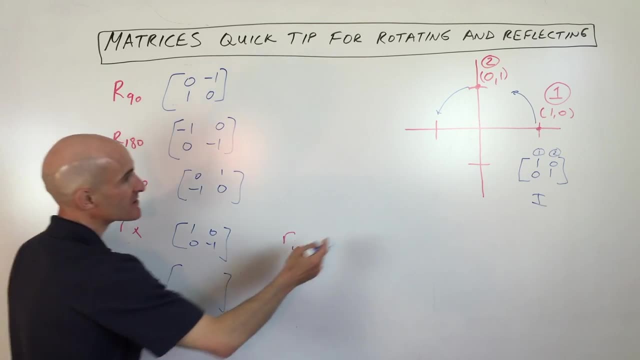 it's going to stay right where it's, at 1, 0,, whereas this point is going to reflect down there at 0, negative 1.. So are you with me? so far? If we reflect over the y-axis, this point's going to. 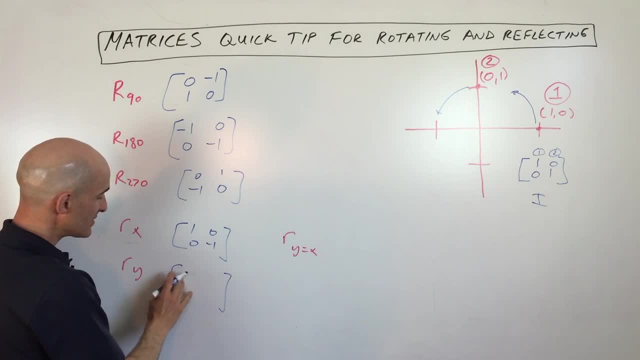 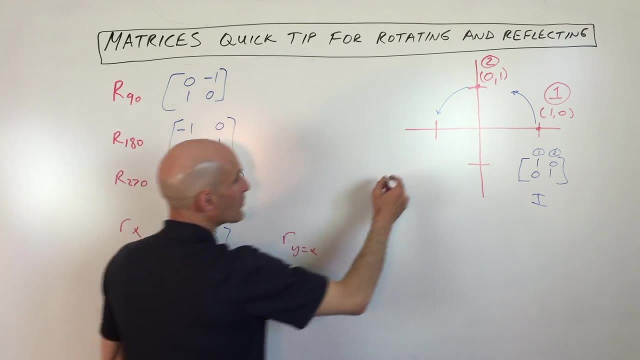 reflect over here. It's going to be at 0,- whoops, I'm sorry, negative 1,, 0, and then this point is on the line of reflection. So it's going to stay where it's at, at 0,, 1, and then the line y equals x. that's this 45 degree. 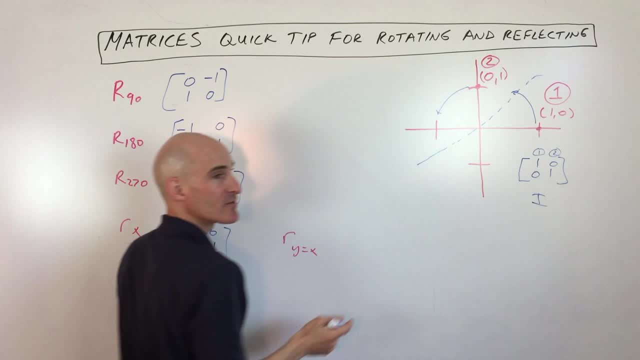 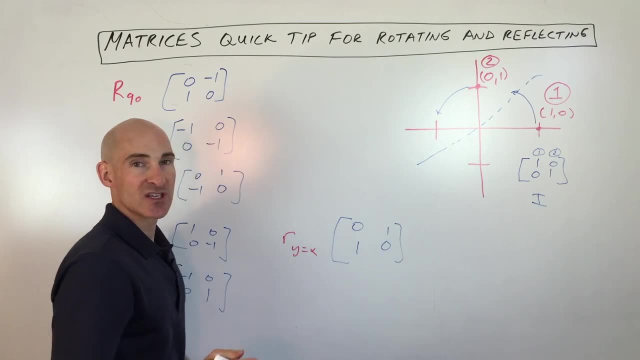 line here. This point is going to be where point 2 is. Point 2 is going to be where point 1 is. They're actually going to interchange positions, so that's going to be 0, 1, and 1, 0, and just to.